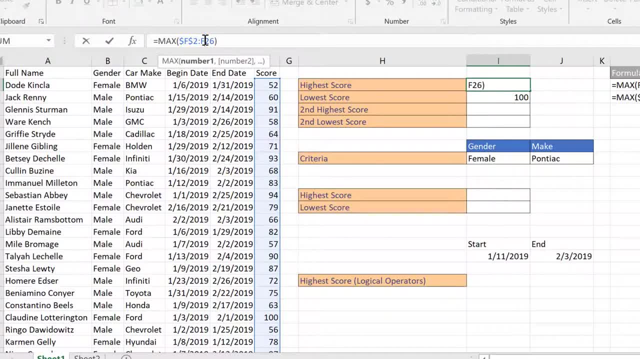 one. Let me show you F4 here and then F4.. Press enter, delete this entry and go here and just bring it down to copy down. And now you'll notice that it stays the same Now with the lowest score. we just use the opposite. 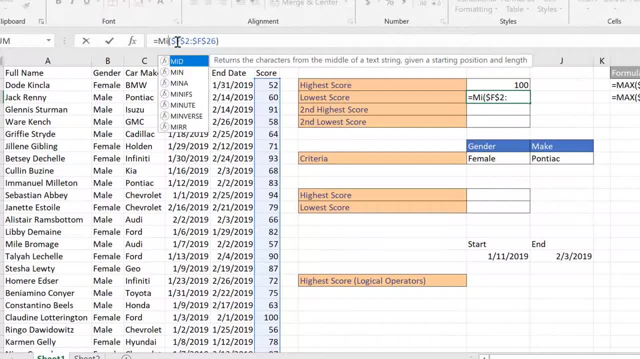 of the max function, which is the min function, M-I-N, press enter and the minimum amount is 52. right over here. How about the second higher score That we can use another function called large, L-A-R-G? Actually, what I can do, since I've got this here, let me just bring it down, since 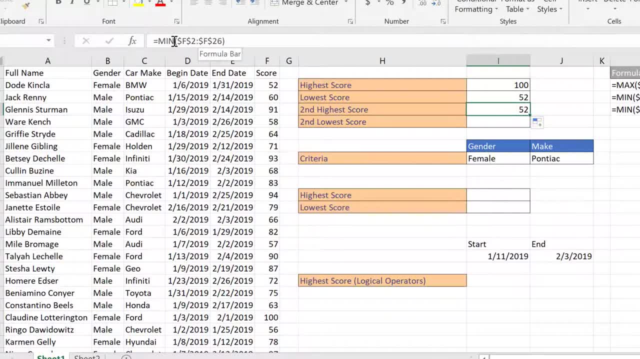 I want to keep that entry here And I'll just change this to large L-A-R-G. Click on that And it takes two arguments. So I need to have a comma. That K is the order, So one would be the first one. If I press one, that's going to be the first, the highest one, which was 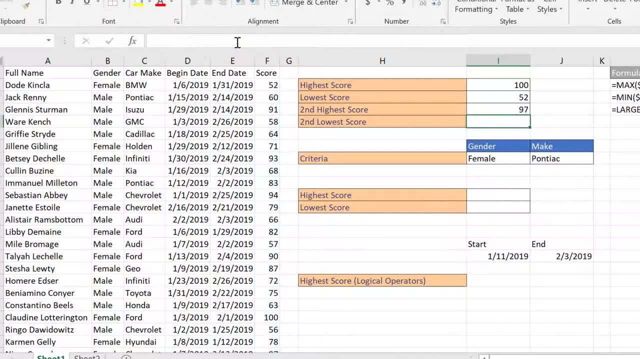 100. And 97 is the second highest here. Yep right there at the bottom. And if we want to do it for second lowest scores, all I'm going to do is just copy that formula down. Since I got my dollar signs in front of them, I have absolute cell references Instead of 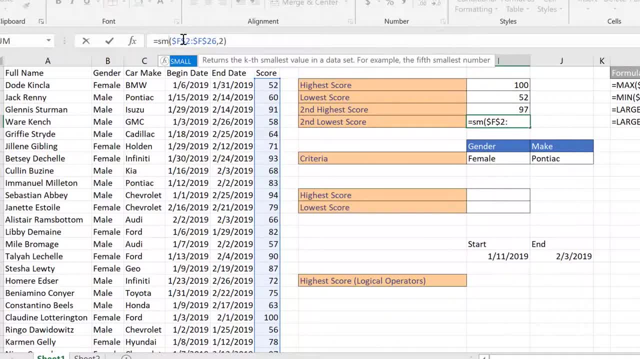 using large, the smallest one, the lowest score. I'm going to use the small function And since I've got the second two there, that's going to be our second lowest score, which is going to be 56.. So that will be somewhere around here, Right, 56 over here. Now, as I 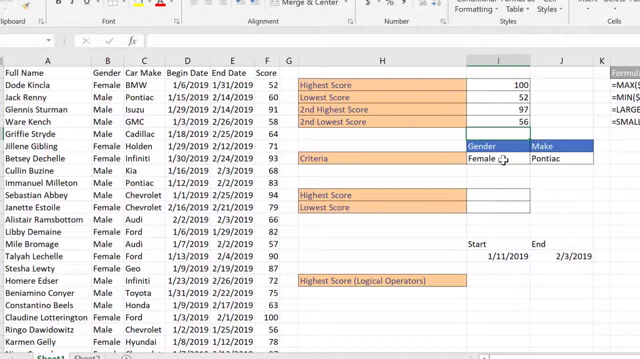 mentioned before, if we wanted to find out using multiple criteria, we would have to use something called the max if functions for the high score And the low score would be the min ifs function. IFS. I'll type equal max ifs. Click on that, It's going to take. 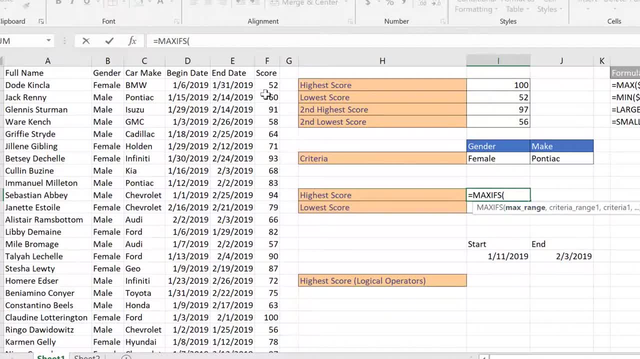 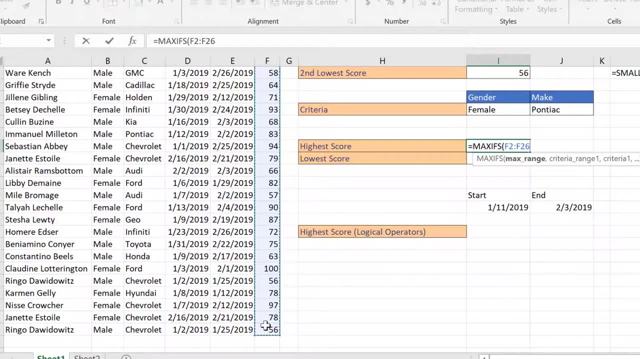 at least two arguments Now. my range that I want to bring back from which is my score range right? Let me select that again And make sure that I have pressed the F4 key And when I press F4, it will automatically. 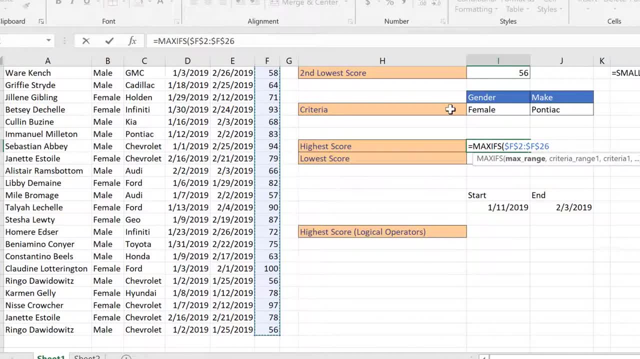 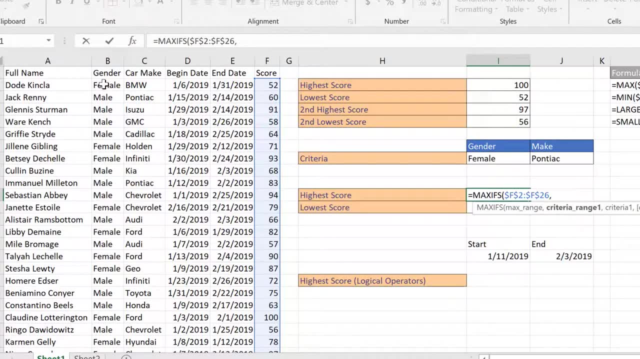 put the absolute cell references for the range here: F2 to F26.. Now, what is my criteria range? So my criteria range, the first criteria: I'm going to select the gender column. So it's going to be B2 all the way down to B1.. 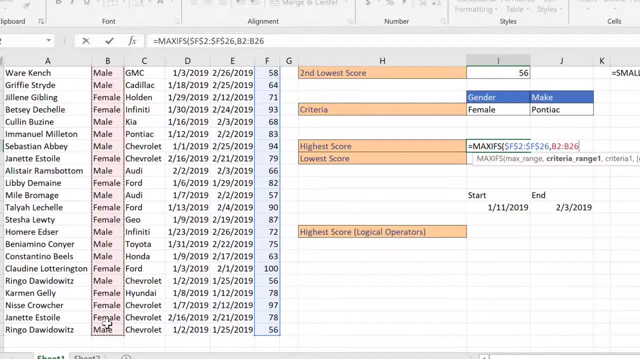 Okay, B2 to B26.. Press F4.. And those are absolute cell references. now, So with that criteria range, what criteria I'm going to use? I'm going to select my criteria dropdown here. So that's going to be I. I also need to press F4 because I want to copy it down to the cell. 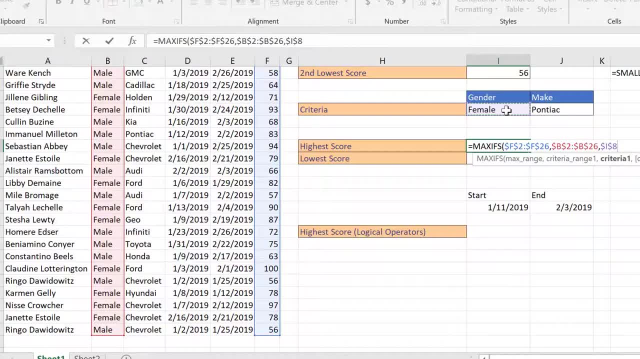 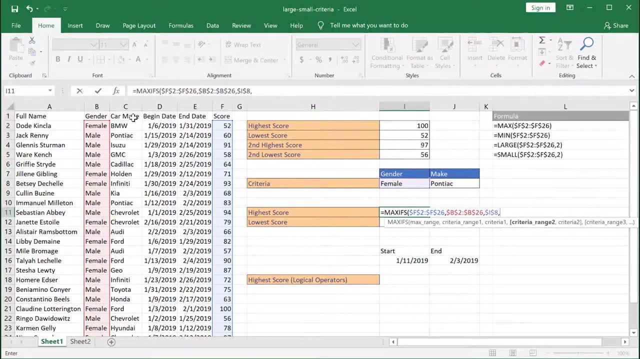 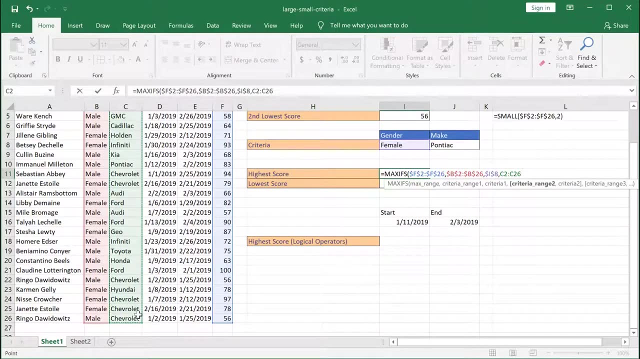 below to the low score section. I don't want that to change either. Comma: What's my second criteria? Well, my second criteria is the make of the car, right. So again, go to make C2.. Go all the way down here And then F4 to lock that in comma. What's my criteria? It's going. 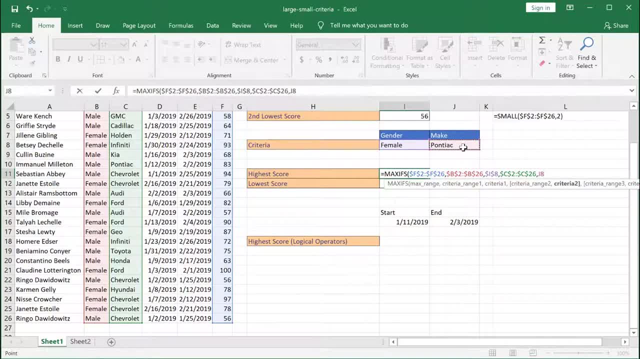 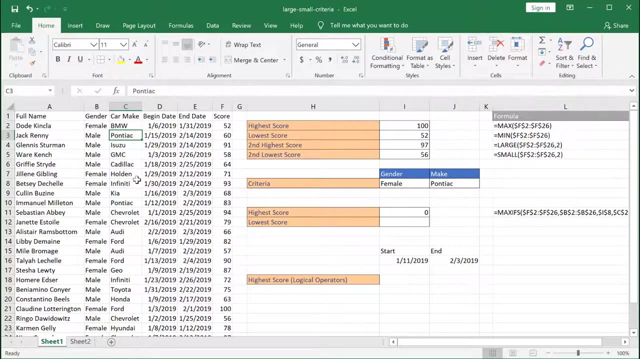 to be cell J8 here, And then of course, F4 to lock that in And close parentheses, press enter and it brought back nothing. So why did it do that? As you can see, there's only two Pontiac entries here: this one and 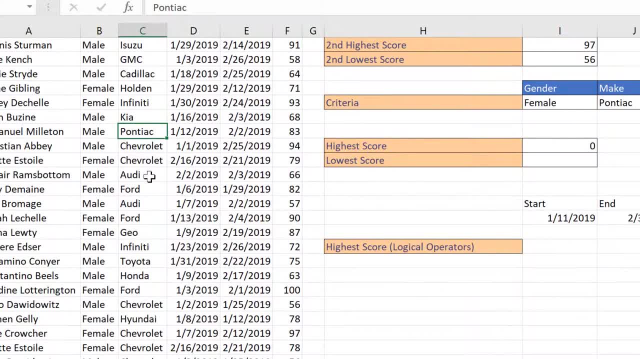 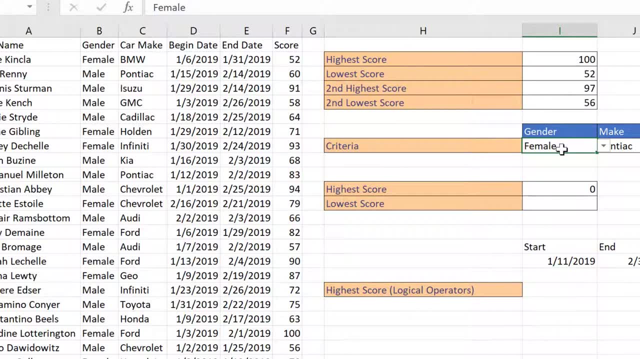 three and this one in row 10 and after that, that was it. so if I change this to mail, I should get an entry back for 60 or, excuse me, 83. so I change it to mail. then I got 83 and that's what happened. alright, so there's the criteria for the. 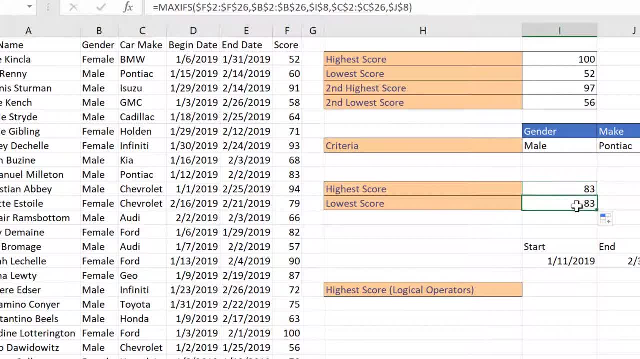 highest now the one for those. I'm just gonna copy that down and change that max if to min ifs and it will give me the minimum min press enter and the minimum for the mail point X, since there's only two to choose from, it's gonna give me 60. 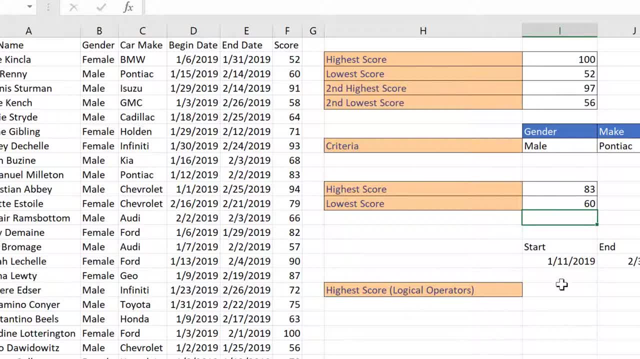 so that's how we can use multiple criteria. now, in addition to the criteria, we can use logical operators if it's higher or lower than so I'm gonna use the start and dates here. now I'm gonna show you how we can do it by putting those dates within the formula and and see what kind of pitfall might happen. 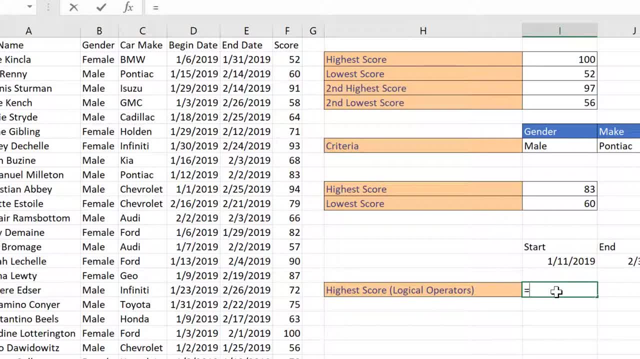 when we do that. so let's just do the high score. I'm gonna do max ifs. press tab the open parentheses and what's my range? I want to do that. so I'm gonna do max ifs. press enter and I'm gonna do max ifs. I want to bring back my scores, select my scores here and I'm not gonna press f4. 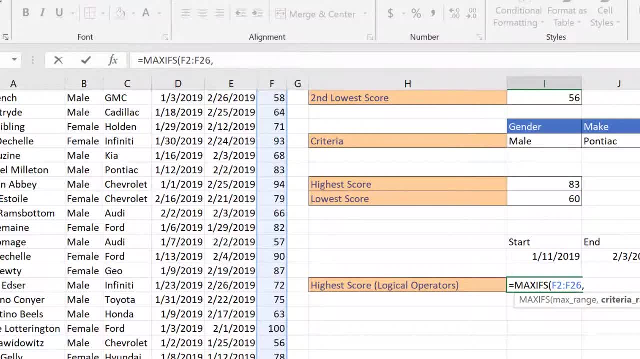 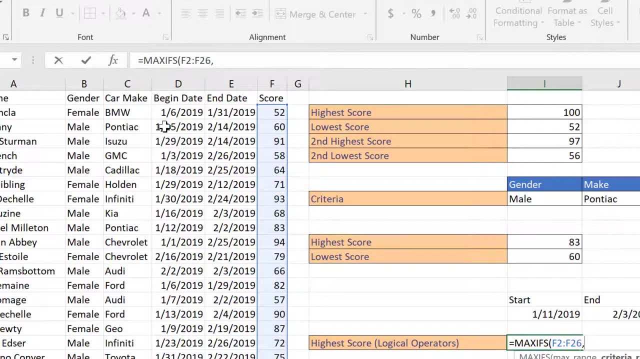 because this is the only entry I've got here, so I'm not gonna worry about copying, pasting it. and with that in mind, what's my criteria range? let's work with our Pontiac entry, since we know there's only two here, so it'd be easier. 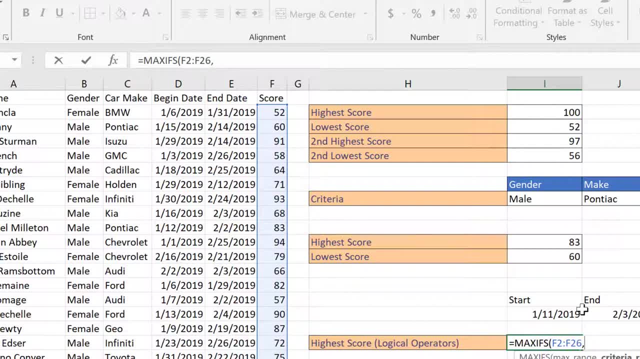 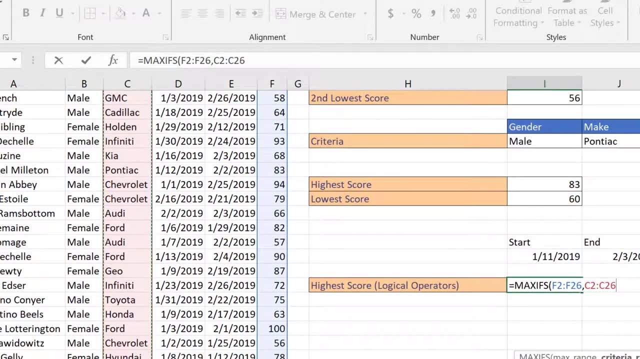 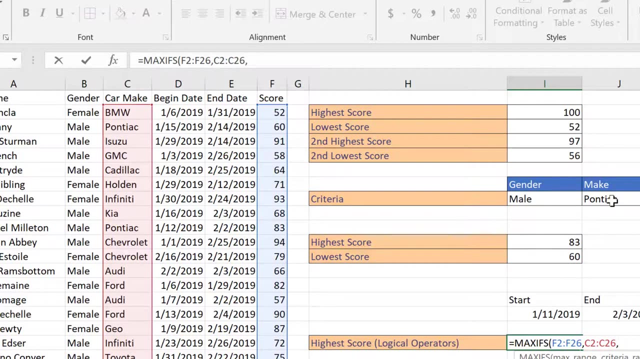 to find out if there's any errors. let's say that I wanted to use my criteria range here and that needs to have that criteria: Pontiac. I can go up here and select it, but I can also put it in here in the entry, so I just have to put it in the quotes: Pontiac, right. 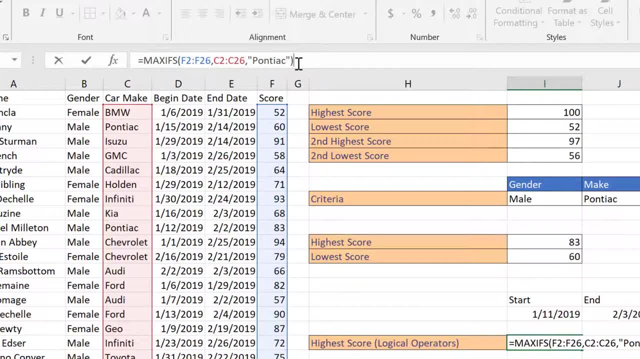 and if I left it as is, it's gonna bring back 83, right, because 83 out of those two is the highest one. but let's bring back some dates, right, let's bring back some dates. let's say that my criterion range, my begin date I'm gonna select. 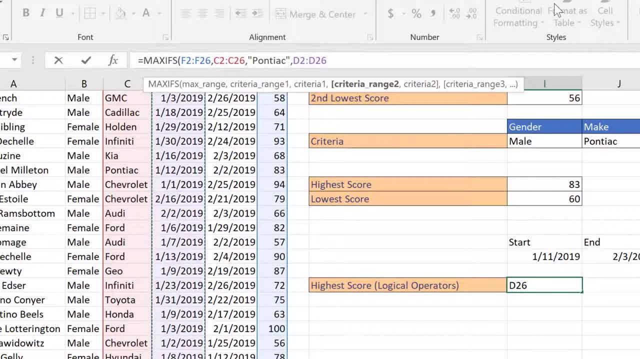 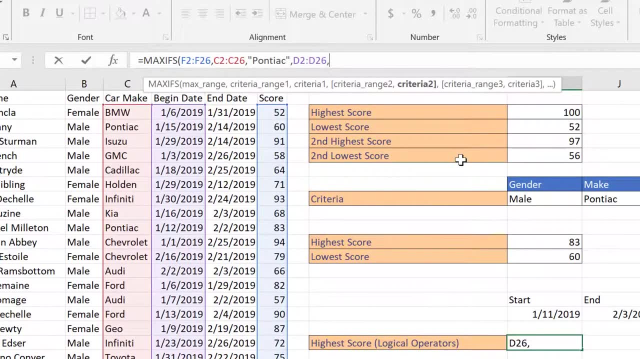 that, that that would be my first criteria, and let's say that I want to have something that is: let's see, we have Pontiac. we don't want it to bring back the max, which was 83, right? so we want to bring back the max that was 60. so the 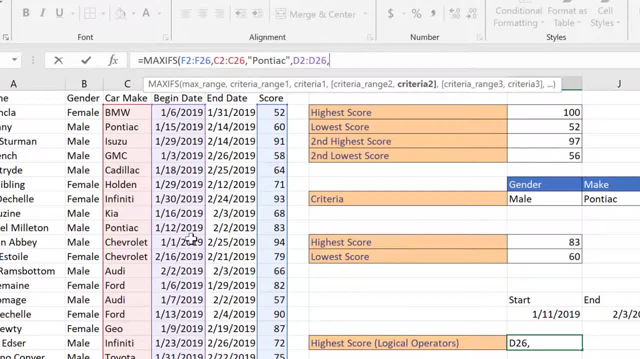 criteria for the date we can say maybe it's greater than January 1st. this entry right here. so what we can do here is we need to put the greater than in the in quotes- so it has to be greater than in quotes- and ampersand it. so we're. 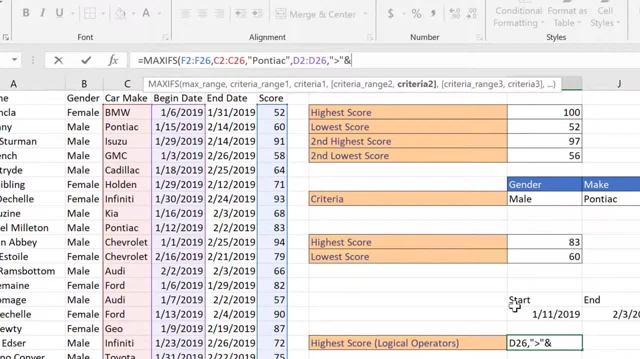 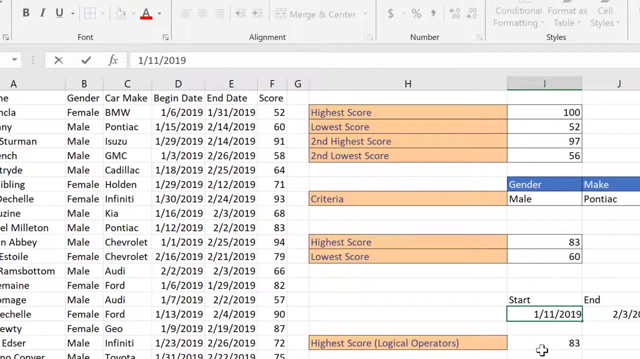 gonna join it. it's greater than that. right close parentheses. press enter. oops, it brought back 83 because the date here, 112 2019, is greater than this one, 111 2008. let's change that to 13. I've changed it to 13, then it's gonna bring. 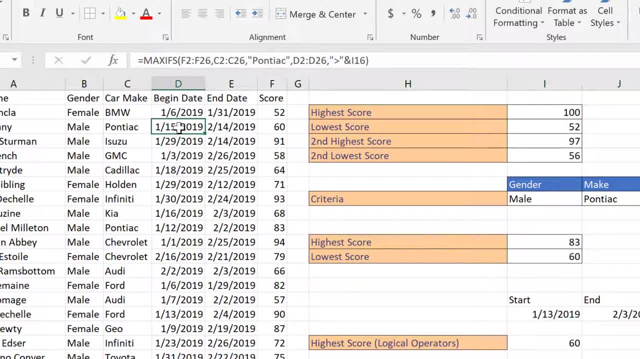 back 60, which is correct because that date is greater than January 13th and that's why I brought back 60. so, as I mentioned before, there's a caveat to this and entering dates. let me copy this ctrl C to copy press escape, if I didn't. 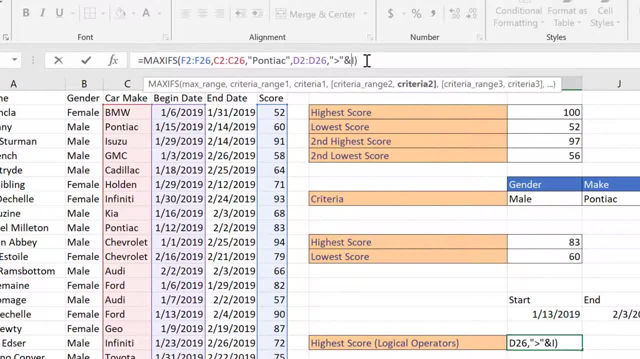 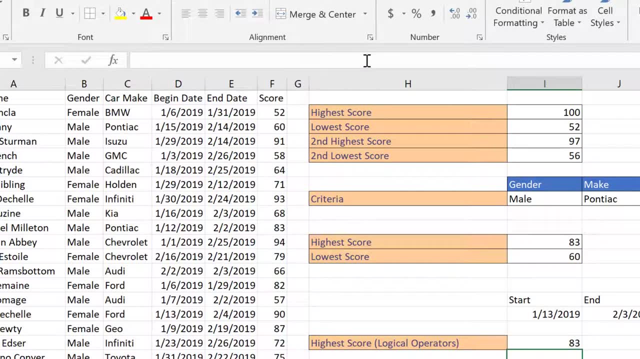 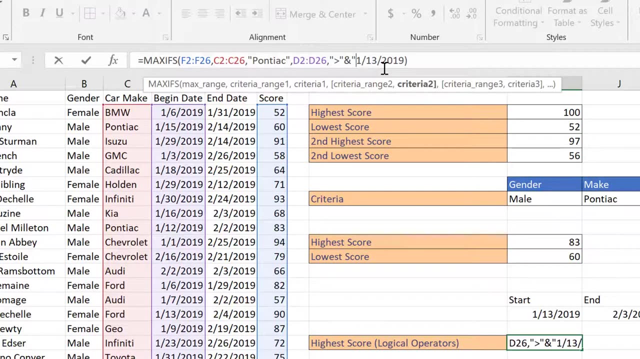 reference 60 here. if I just said, if I said, if I said command V, control V, to put that in, if I'm going to reference the date here, it's not going to work, it's going to. it won't work correctly, right, but I think if I put it in quotes, let's see Excel might be smart enough to. 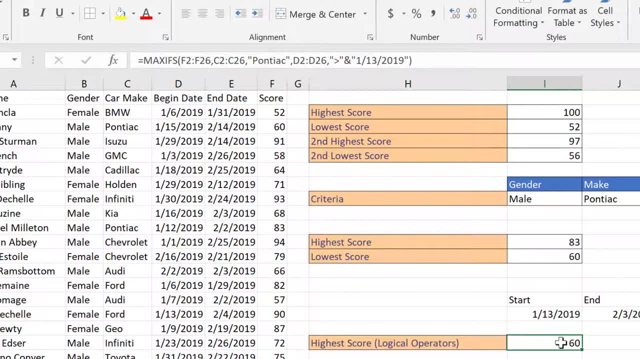 recognize it, yes, and then it brought it back correctly. so there's the various ways that we can use criteria to get our smallest and largest values. now, as I mentioned before that, I can show you how these drop downs are created, and it's actually fairly easy. all I need to do is, if I 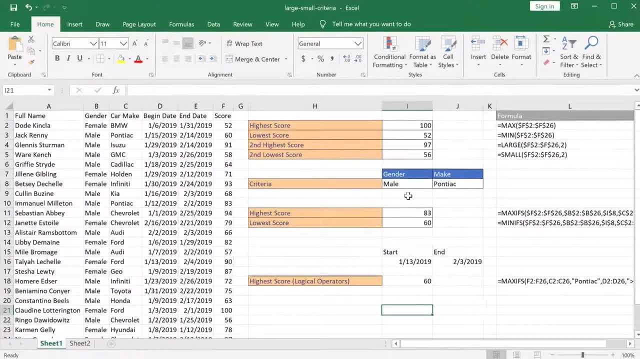 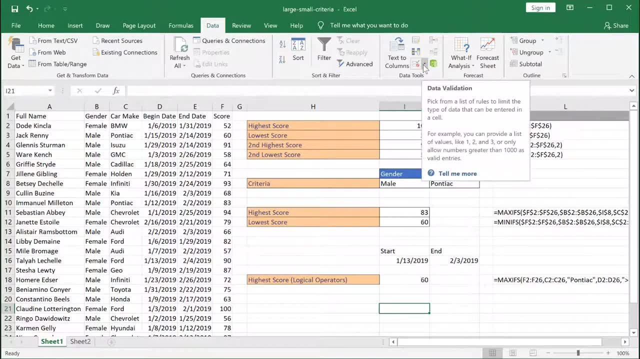 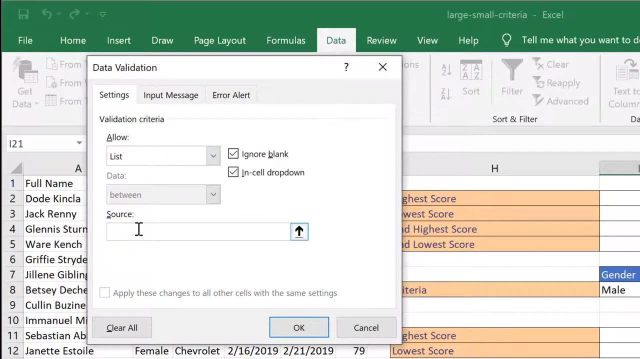 create a drop down like that one. we're only, there's two entries, there's not that much typing. this is the data validation list, so I'll just go under data and go to my data validation, click on that allow, click on list and here I'll just type out the two entries. it's either going to be a male. 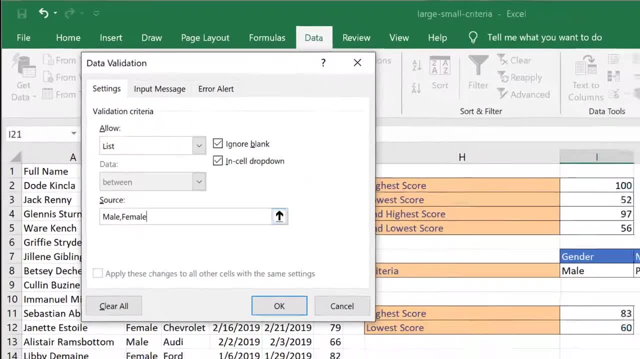 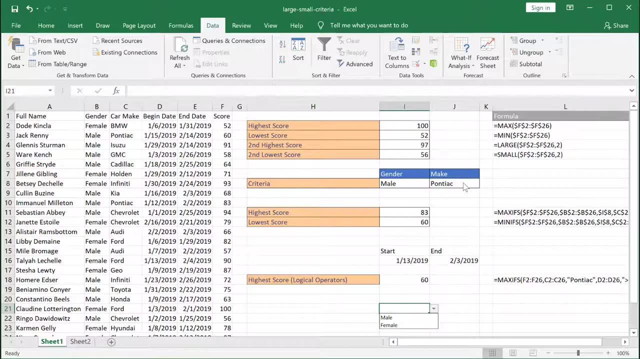 or female, click OK and now I have my drop down- male or female- with the other drop down. it's a little bit more challenging because we have more than one, more than two entries. maybe three or four is easy, easy to type in, but if you've got quite a few you don't want to type. 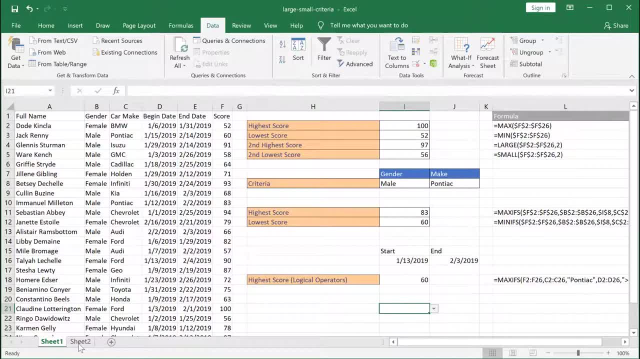 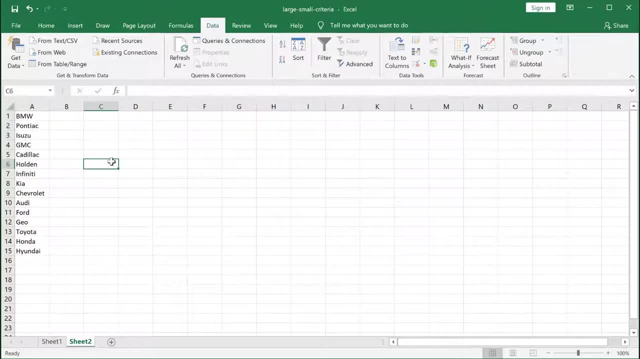 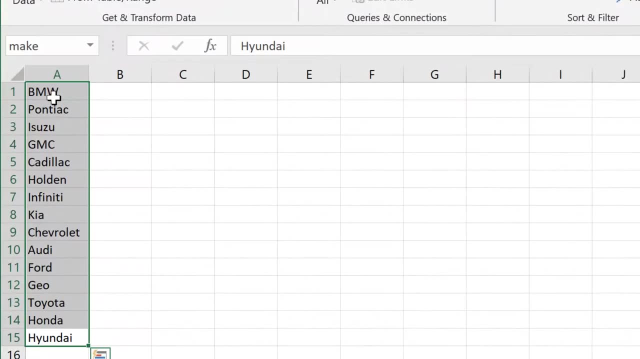 in all of those, so we need to take that and put it into a column. I already have a column here and we have our 14 uh makes here and what I need to do is make sure that this is a named range. this range is named. I'll just copy this, because I already named this one earlier. I'll put it over. 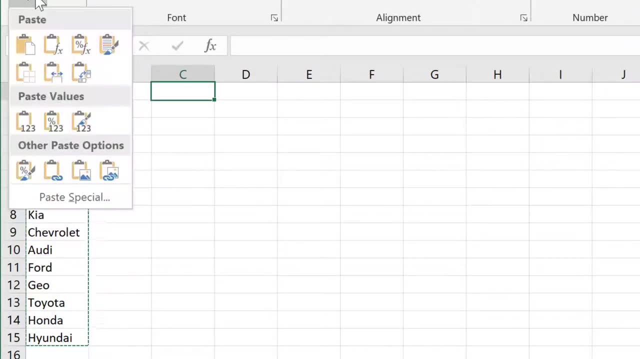 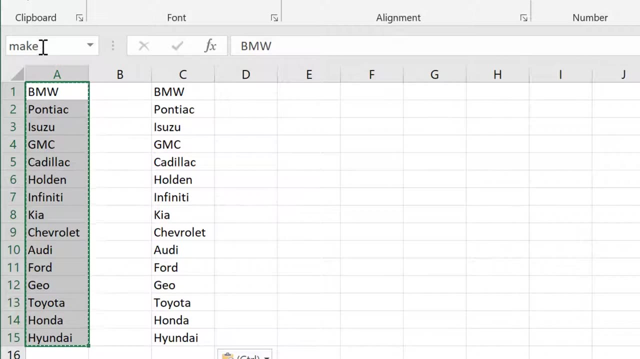 here and I'll paste just the values, so hopefully I don't paste the name range there too. and this doesn't have a name range. you can see, if I select this over here, there's a name here, but if I select this, there's no name. so and I'll just call this one, make two, the second one right, and so I've named.